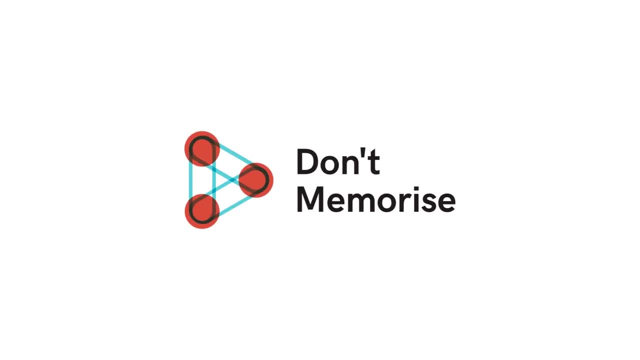 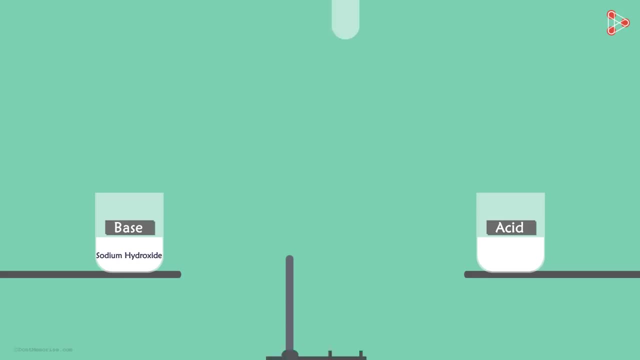 To understand how acids react with bases, we take about two millilitres of sodium hydroxide solution in a test tube and add a couple of drops of phenolphthalein solution to it. What do you notice about the colour? Yes, the colour of the solution turns pink. The indicator phenolphthalein is colourless in acidic solutions but goes pink in basic solutions. As sodium hydroxide is a base, the indicator turns pink. Now to see how bases react with acids, we add hydrochloric acid to this drop by drop. What do you observe? We see that the solution turns colourless again. So the colourless base turned pink and then again turned colourless after an acid was added. What does this prove? We can say that the effect of a base is neutralized or nullified. 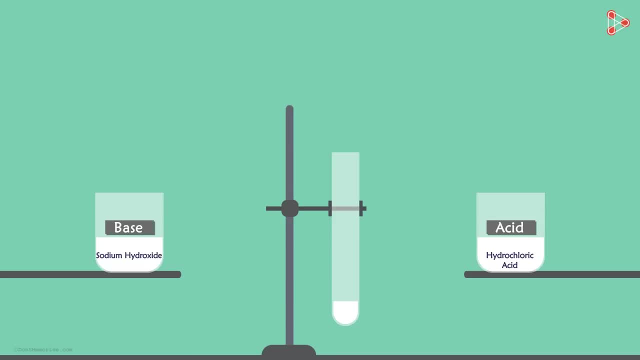 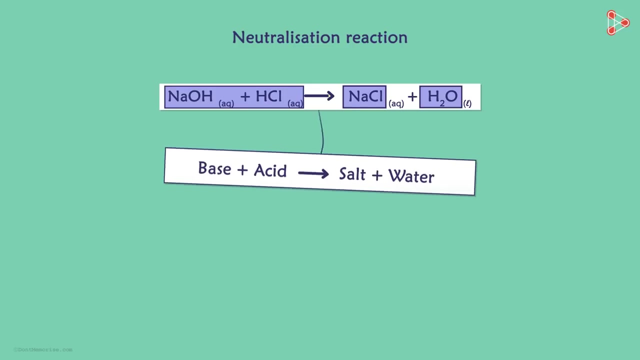 Does the reverse also happen? Will an acid be neutralized by a base? To find out, let's add a few drops of sodium hydroxide back to the above mixture. And yes, the pink colour of the phenolphthalein reappears. That's because the effect of acid is neutralized by the base. So the reaction taking place here can be written like this. Sodium chloride is nothing but a salt. So when an acid and a base react to give us salt and water. And guess what such a reaction is called? It's called a neutralization reaction. A base reacts with acid to give us salt and water. In a similar way, calcium chloride is formed along with water when hydrochloric acid reacts with calcium hydroxide. 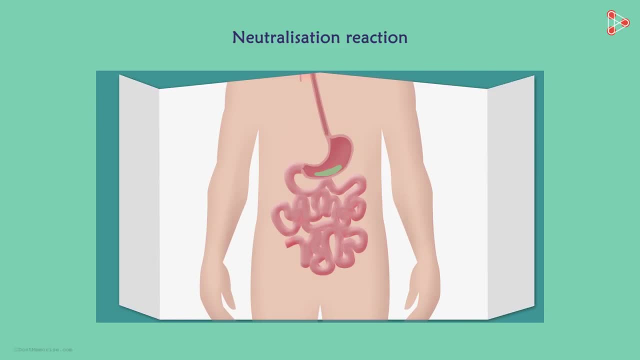 Can you think of a more practical reaction? When we have acidity, our stomach produces excess acid which is nothing but hydrochloric acid. So what happens when we have acidity? When we have acidity, our stomach produces excess acid which is nothing but hydrochloric acid. When we have acidity, our stomach produces excess acid which is nothing but hydrochloric acid. 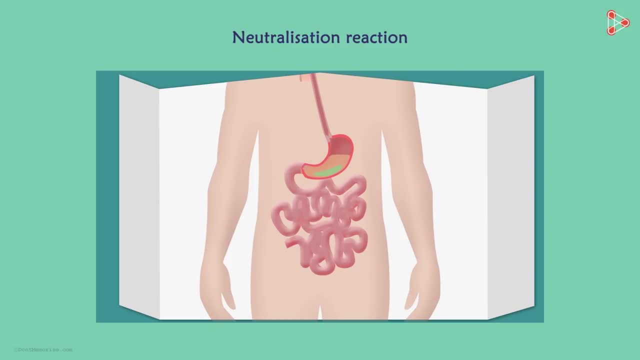 And this acid is very harmful for the walls of our stomach which is why we get that burning sensation. So to neutralize the acid, what we use is an antacid. Antacids as you would have guessed are nothing but bases. The antacid reacts with the base to give salt and water. And that gives us relief!